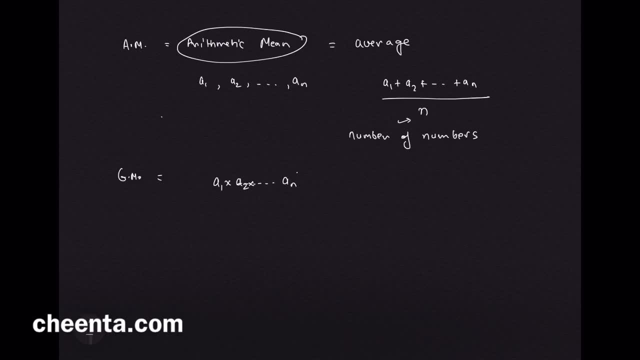 numbers: a1 times a2 up to an and you raise it to the power 1 over n. So this is simply the nth root of the product of all the numbers. Now the question is: is this well defined? Is this well defined? And you can readily see the problem. 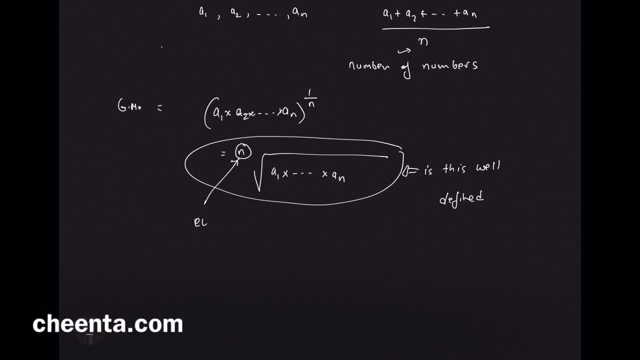 I mean, if n is even and if some of these numbers is negative, then there is a possibility that the product of these numbers is also negative. If the number of numbers are negative, then certainly the product will be negative In that case. and if the n, if n is even, then you cannot really take the nth root of it and get a real number. 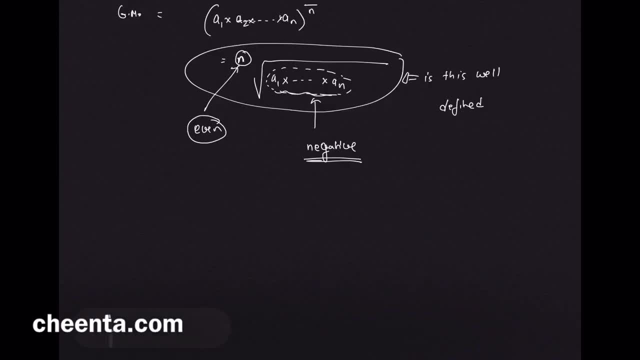 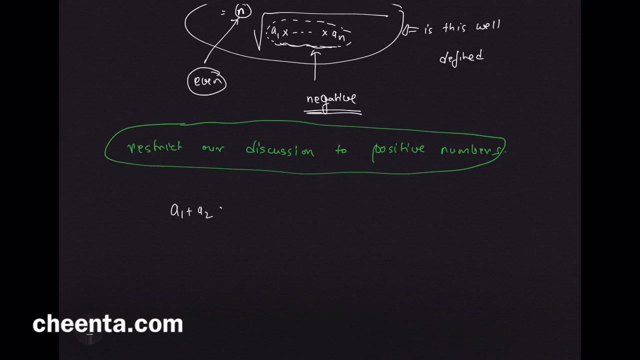 So what we do is we restrict ourselves, restrict our discussion to positive numbers only. Okay, So that will make both of these quantities well defined and we can compare them. There is a very well known algebraic result: that the arithmetic mean, that is, the average, is greater than or equal to the geometric mean of these same set of numbers. 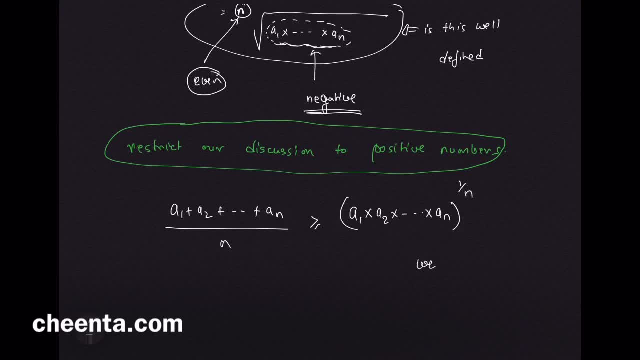 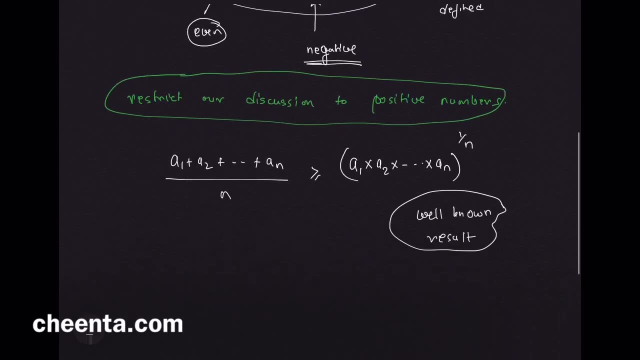 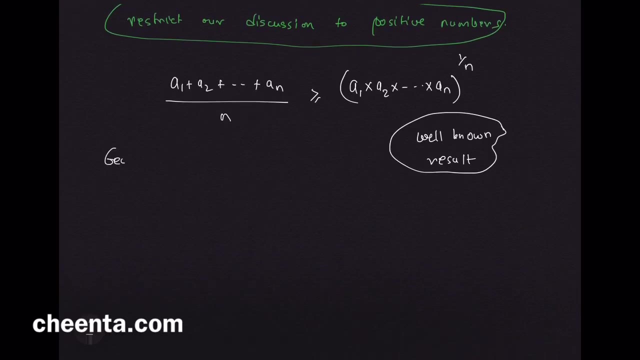 So this is a well known result And we will not look at the, the proof of this today. this: this can be done in the in our class, but today we want to look at a geometric interpretation of this. a geometric interpretation and really we want to look at two quantities, so a1 and a2, and 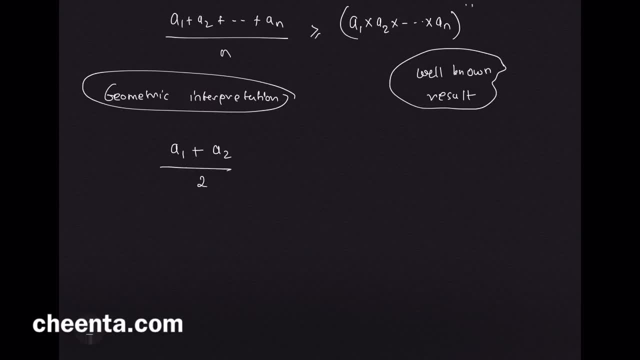 their arithmetic mean is simply their sum divided by 2 and their geometric mean is: you take the product of the numbers and raise it to the power half. and remember a1 is greater than 0 and a2 is greater than 0. we are only dealing. 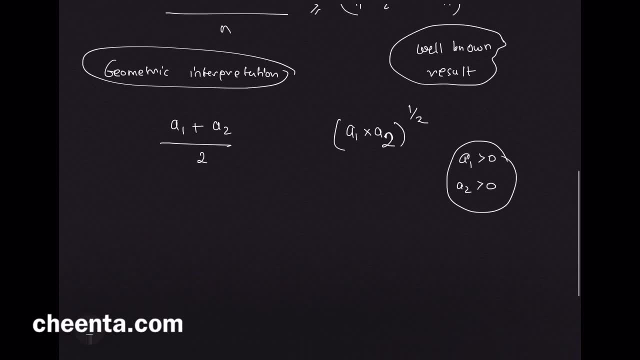 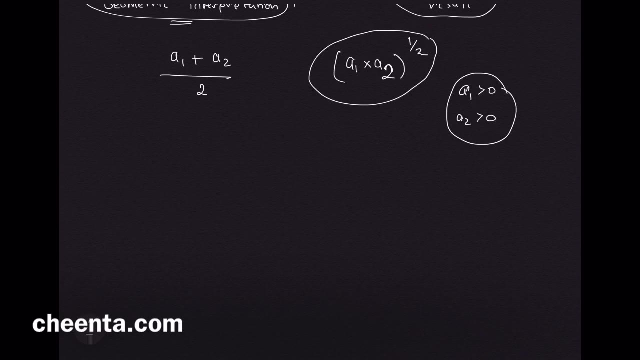 with positive quantities, and this can be extended, but let's focus only on positive quantities for the moment, just for fun. okay, so we have. we want a geometric interpretation of this. but first let's look at how can we construct the square root of 8: a 1 times a- 2. 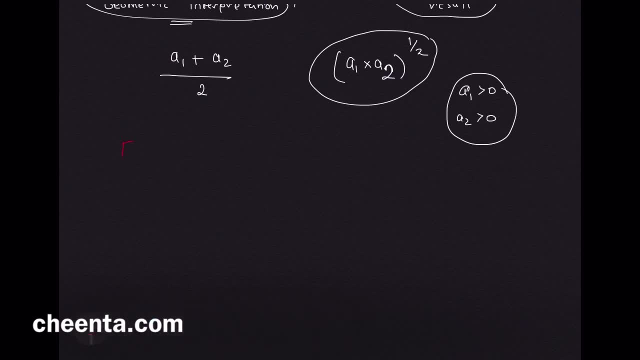 so this is? this can be a little exercise and you can look in the link in the description. it will take you to a small quiz which will help you to solve this problem. so what is this? we want to construct the square root of a 1 times a. 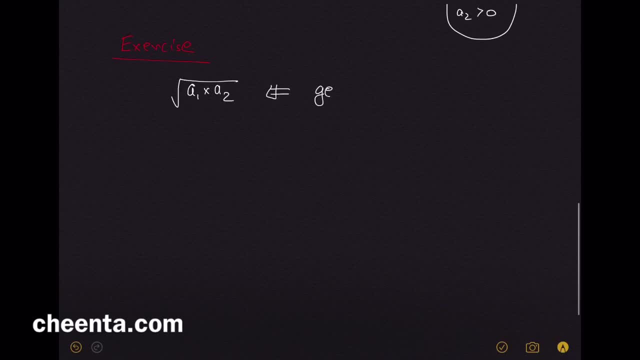 2 geometrically. so, using a compass and pencil and maybe a straight edge, can you construct the square root of a 1 times a 2. suppose a 1 is 3 and a 2 is 5. can you construct square root of 15 using? 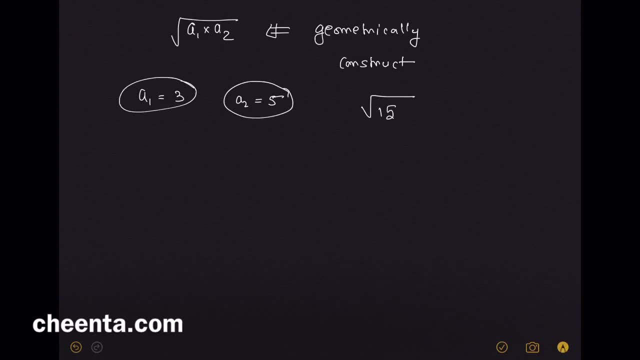 a compass and a pencil and a straight edge. well, this is how you can do it. take a unit 3, 3 unit long, 3 unit long segment, let's call it a, B, and take another segment and that segment should be 5 units long. so here you go: 5 unit long. let's call this C, 5 unit long. and now. 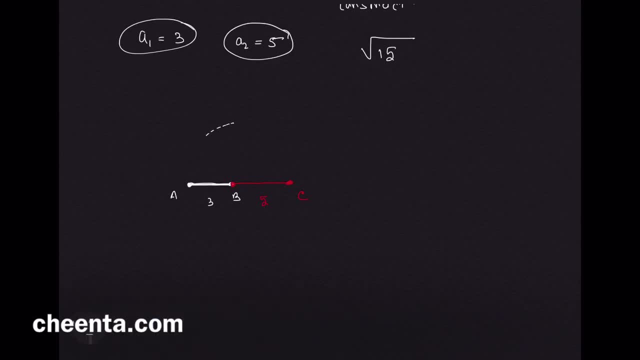 take a circle. take a circle like this and this circle is off radius. it should have AC as the diameter. AC is the diameter of that circle and that means the radius is 3 plus 5 over 2. notice that the radius is the arithmetic mean. is the arithmetic mean of these two numbers. so you can take the midpoint of. 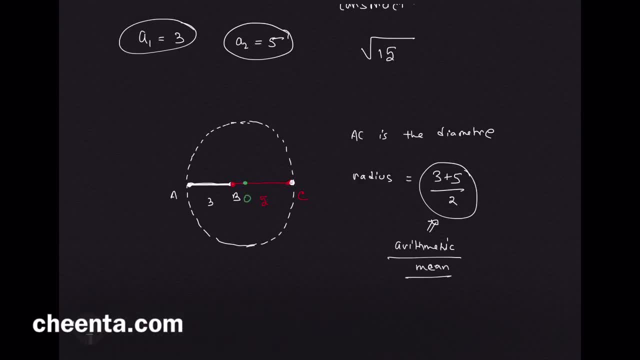 this, let's call it O. then OC is the arithmetic mean of these two numbers that you started off with: 3, 3 and 5, and if you erect a perpendicular at O, let's call it OM. this is also the radius. so 3 plus 5 over 2, that's the value of the. 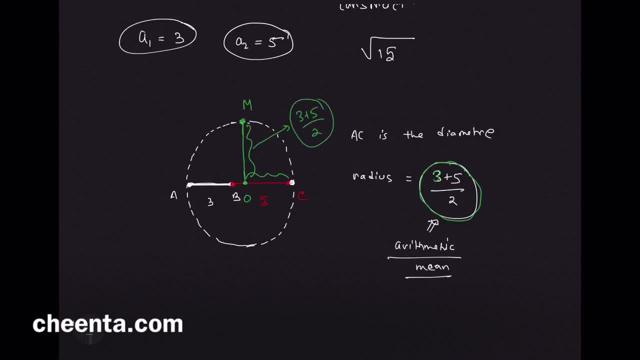 radius. simple enough. the crazy part is this: if you want to find the geometric mean, all you have to do is to erect a perpendicular at the point B. erect a perpendicular at the point B, so this quantity will happen to be square root of 3 times 5. why can you prove this? 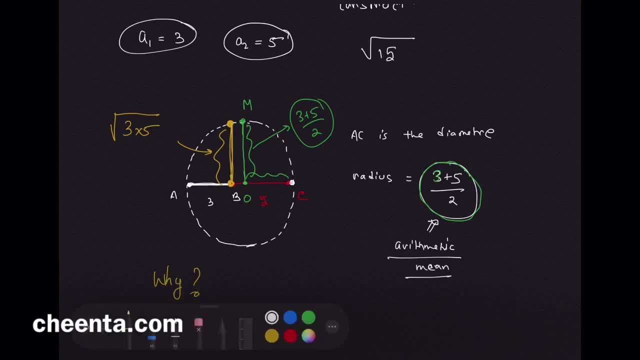 well, I'll give you a hint, and more hints will be in the link in the description. but this is how you can go about it: join. so let's suppose this point is: n? join a, n and c? n. join a, n and c? n. now can you show that triangle a, b, n is similar? 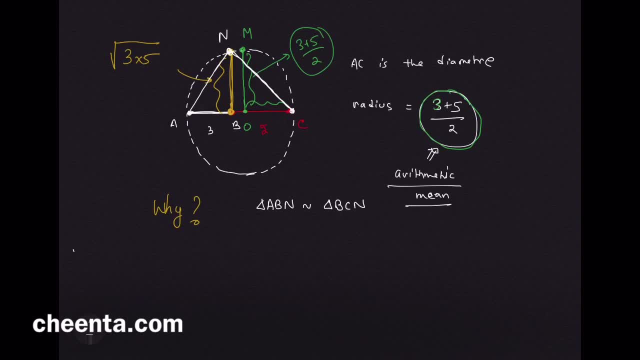 to triangle BC n, and that's similar to triangle a and c. that is all. these three triangles will be similar to each other. it's a very important and well-known result in geometry. now, using this result, you can show that B? n is indeed square root of 3 times 5. 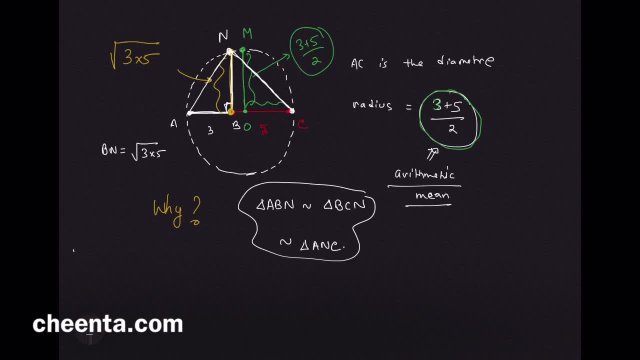 now, if this B, n is the geometric mean and if OM is the arithmetic mean, you can easily see that the radius will be greater than any other half chord, right? so if you look at this B and you can talk, think of this as a half chord. so B. 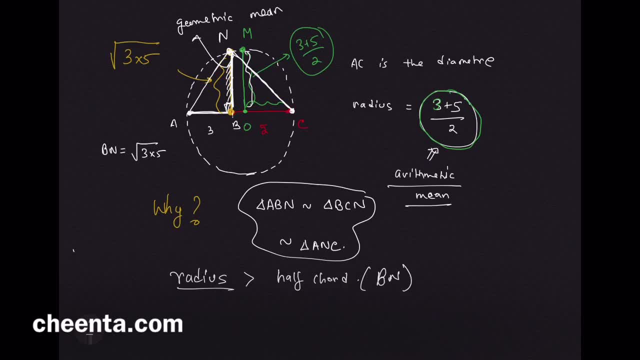 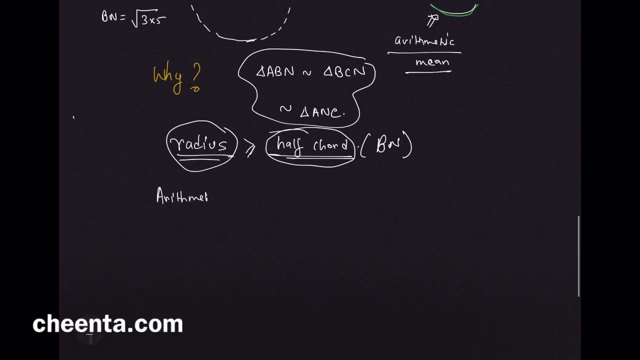 in this case B, and is the half chord. radius will be greater than or equal to any other half cord in this particular circle. that's because diameter is the largest cord inside the circle. so the fact that radius is greater than any other half chord translates to arithmetic mean is greater than or equal to the geometric mean. this is wonderful. 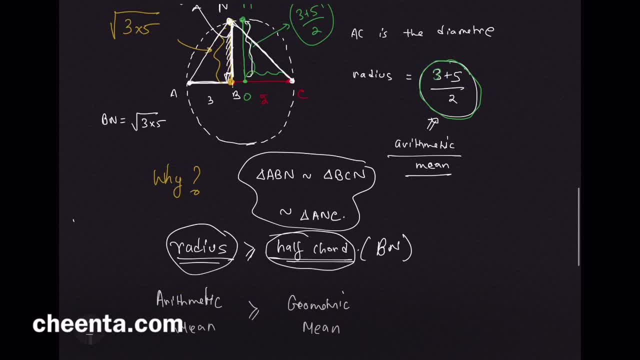 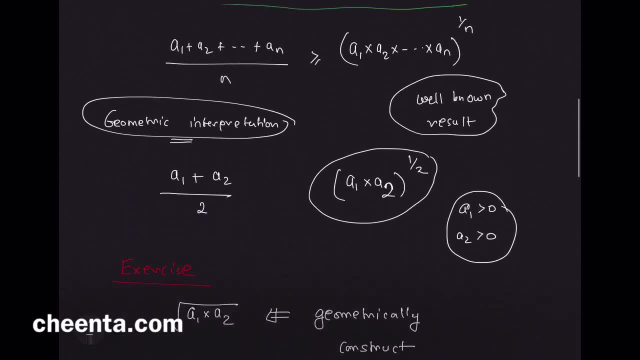 right. so can you show this rigorously that B: n is indeed square root of 3 times 5? and then you have finished this construction with the proof. all right, keep on doing wonderful mathematics. we will meet soon again in the next video.